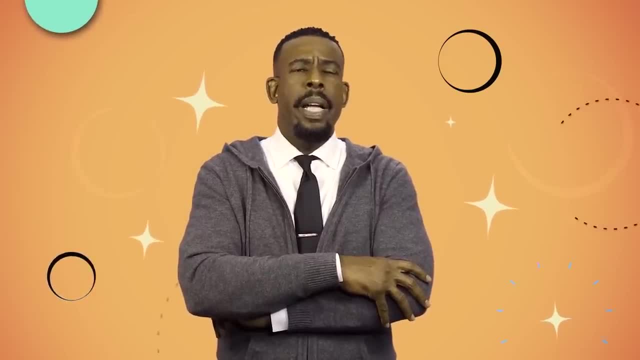 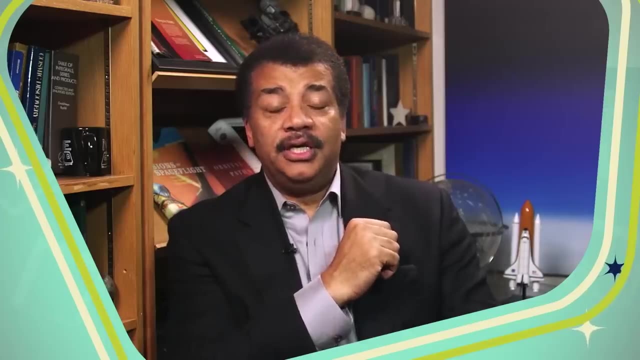 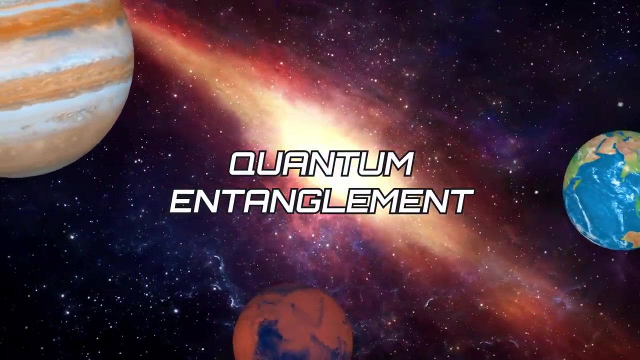 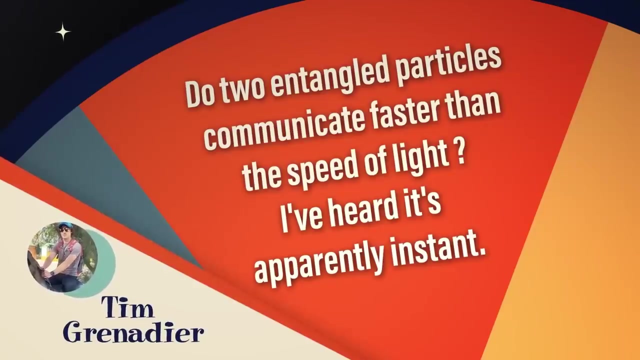 So what party is it where you sit home and lament your career and cry? What particle is that? That's the neutron. It has no charge, so therefore it can attract no one. Tim Gurr says: do two entangled particles communicate faster than the speed of light? 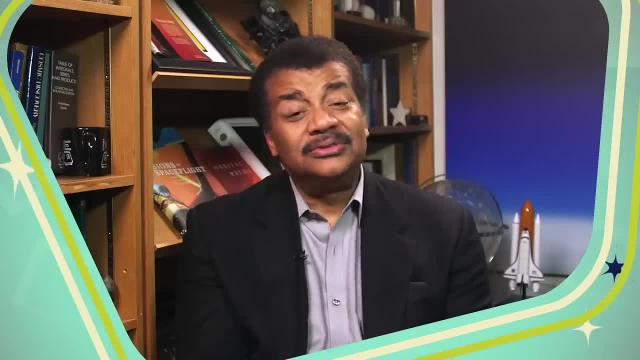 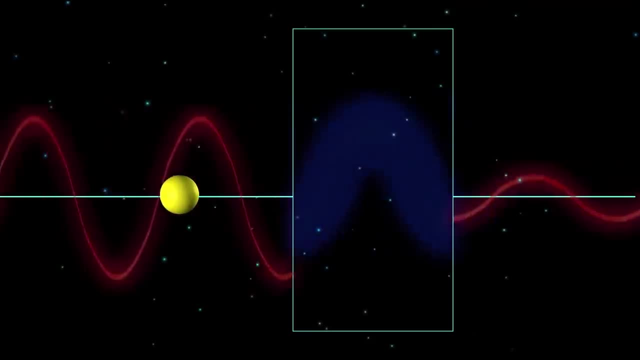 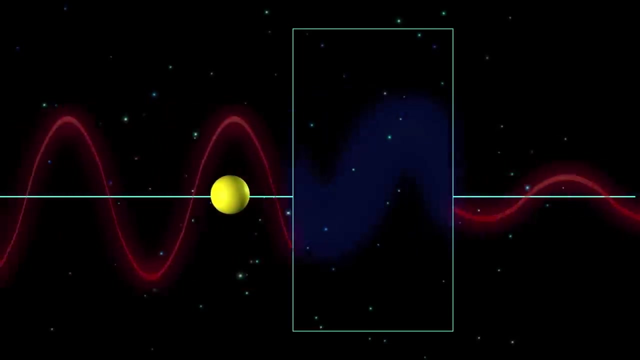 I've heard it's apparently instant It turns out. one of the rules of quantum physics is that, because particles are also waves, if there's a particle on this side of a hill and it can't get across to the other side, the wave function does exist and actually exists in a little bit on the other side of the hill. 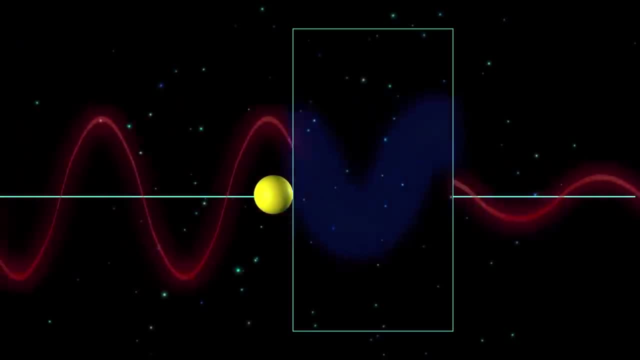 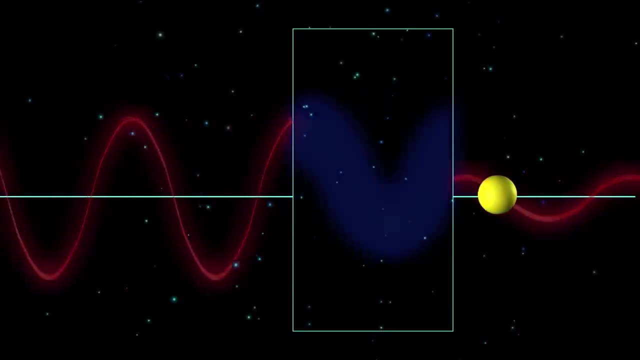 So the electron can disappear here and reappear there, collapsing the wave function and the electron would have moved from there to there instantly, Basically faster than the speed of light. It's called quantum mechanical tunneling and it happens all the time. 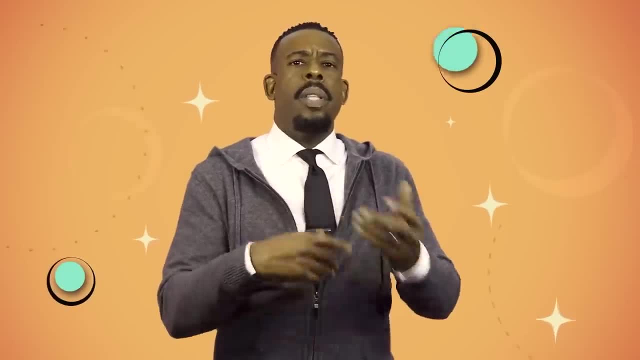 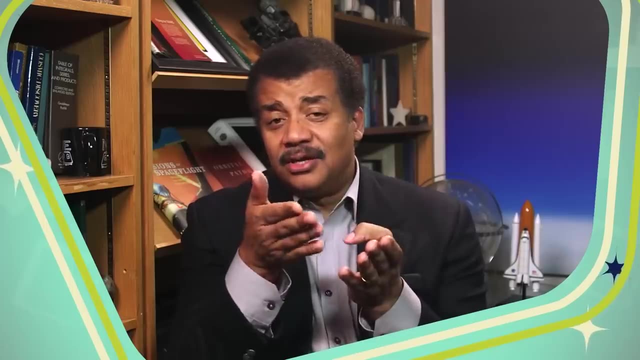 And it is mysterious and beautiful. So what's the hype about tachyons then? So tachyon is a hypothetical particle named for being very fast. Tachyos is Greek for speed. The tachymeter gets the same root. 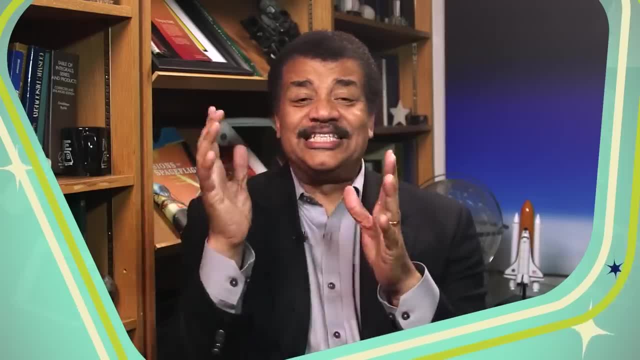 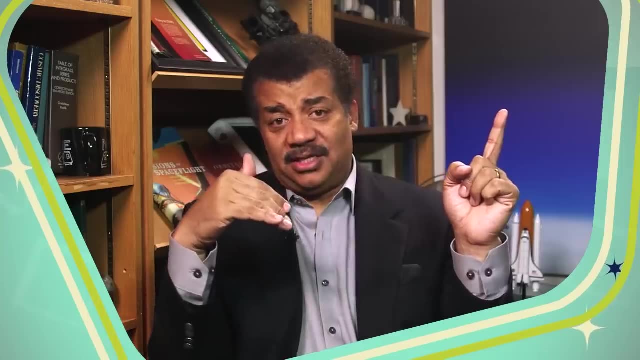 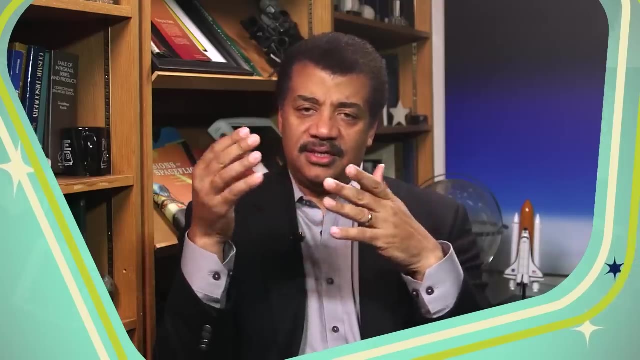 So a tachyon is a particle, a hypothetical particle, that exists only faster than light And it can go to infinitely high speeds, And the slowest you can ever get this thing to go is the speed of light itself. It turns out this is not violated in Einstein's equations. 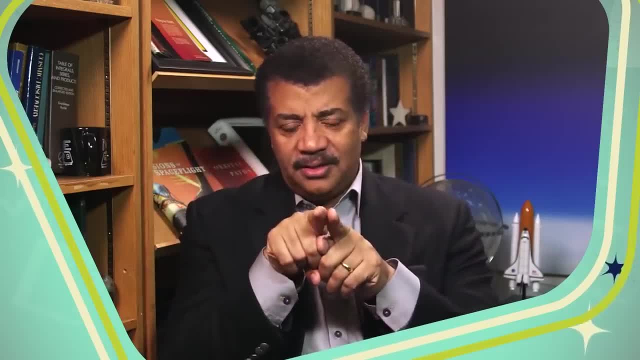 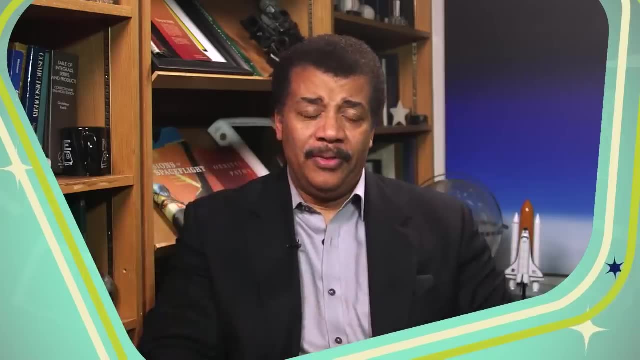 because you're not crossing. You're crossing the speed of light. You're coming into existence faster than the speed of light And you put that into the equations, it ends up living backwards in time. This is a backwards, time-traveling particle. 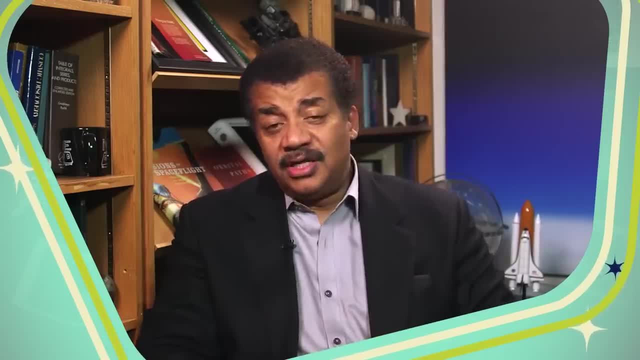 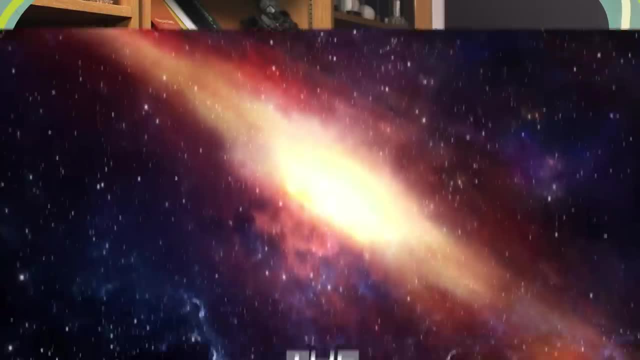 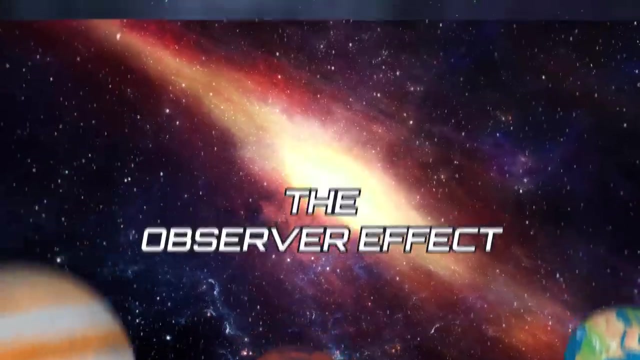 Hypothesized. we've never discovered one, So we don't know if they really exist. They probably don't, but it's fun to talk about them because they don't violate Einstein's relativity equation, And that relates a little bit to what people have called the observer effect. 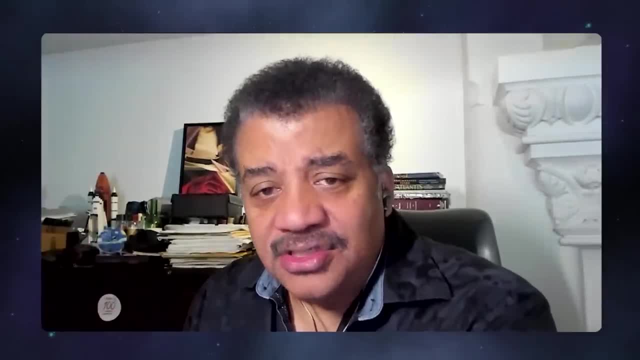 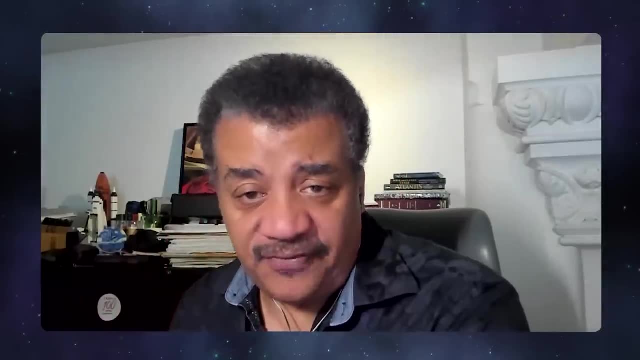 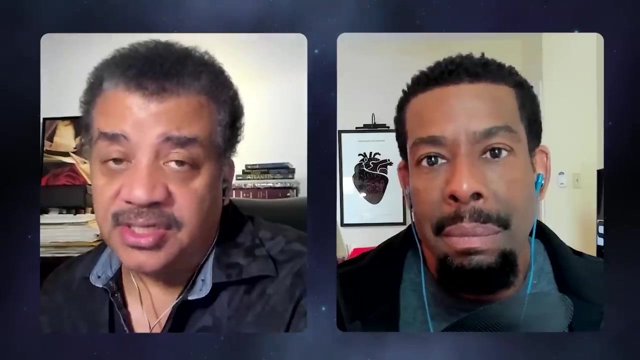 Where if you observe something, you change it. So I can respond to both of those in the same pop, if you allow me. So let's do the observer effect for the moment. So it's unfortunate that somebody called it the observer effect, because then New Age folk and other people who were basically scientifically illiterate- 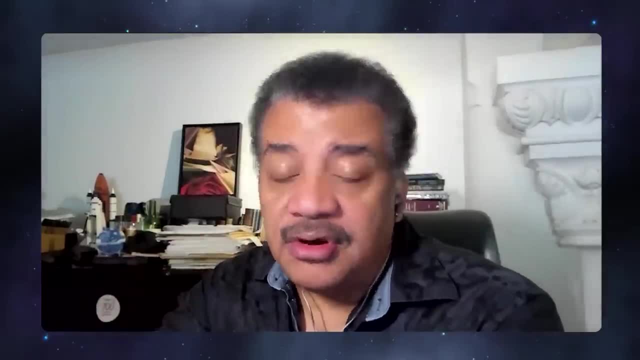 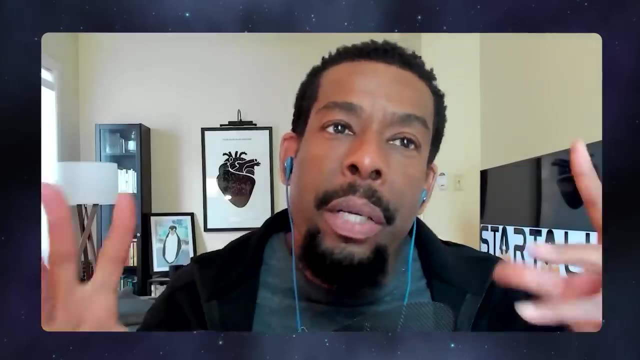 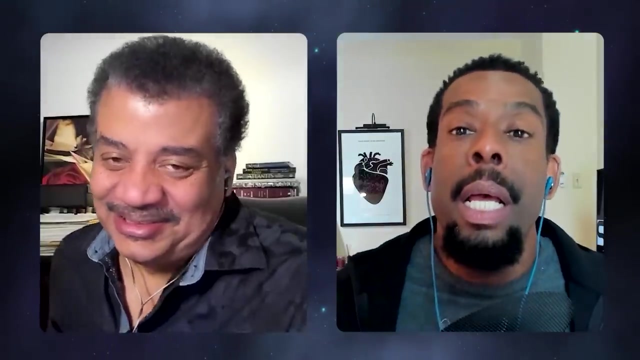 were thinking it's your consciousness that affects what you're observing And, oh my gosh, there's a consciousness field And they go running off the cliff. See, what you don't understand is that particles are totally alive And the reason why there is a collective consciousness in the universe. 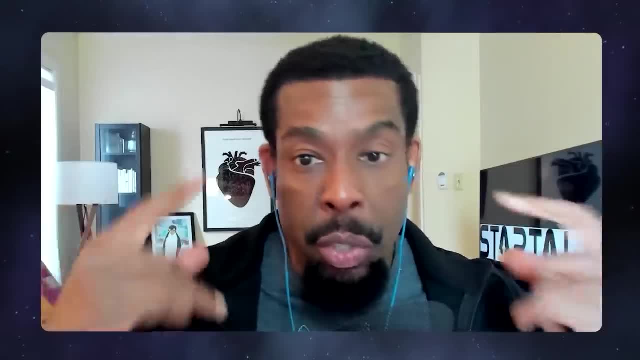 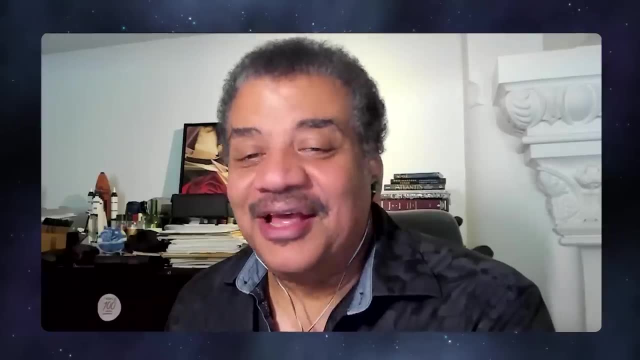 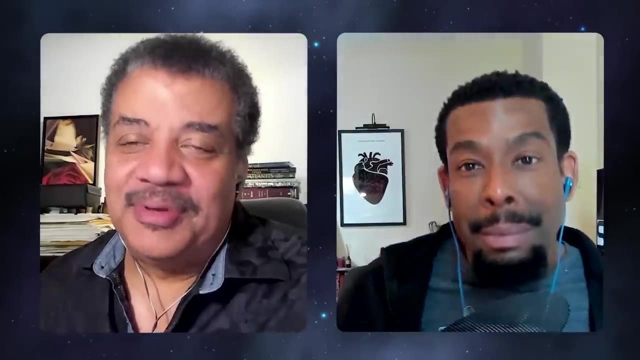 is because all of these particles that are spinning, what they're actually doing is conducting thought and consciousness. They're thinking. They're thinking man Rocks think, Trees think Yeah, More than rocks, Right? So let me cut through all of that and simply say that you're sitting there. 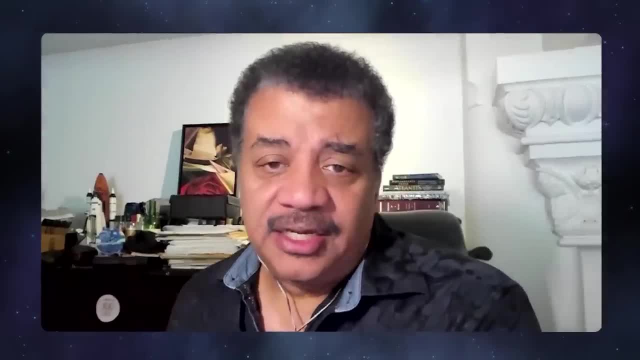 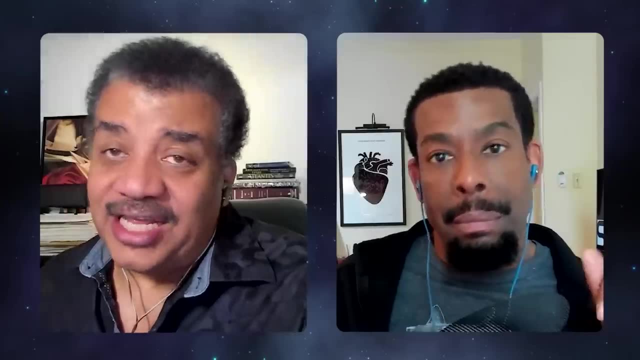 and I can see you because, in fact, you're illuminated by, if not sunlight, through an open window, an uncurtained window, but artificial light within the room. All right, That light hits your face, bounces off your face. 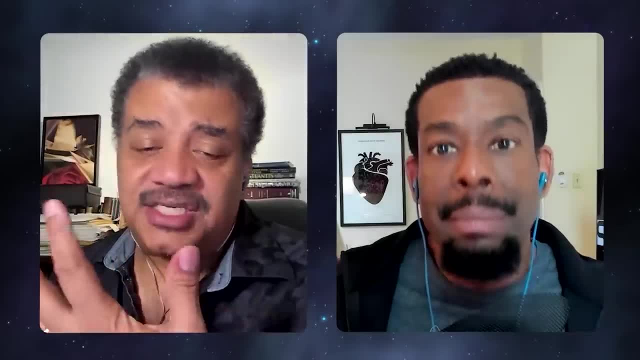 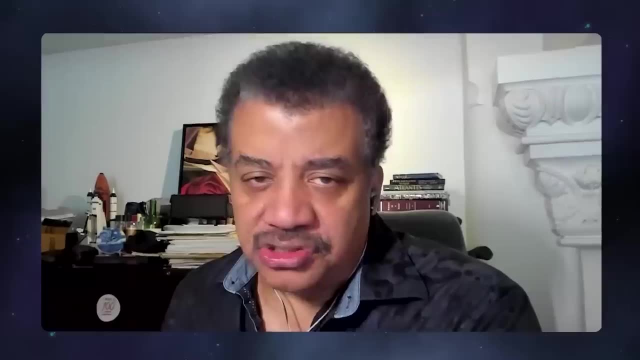 goes through the computing system and I see you. Okay, That light carries energy. Every photon of light that strikes your face carries energy And most of them reflect. Others get absorbed. Actually, it depends on how dark your skin is. 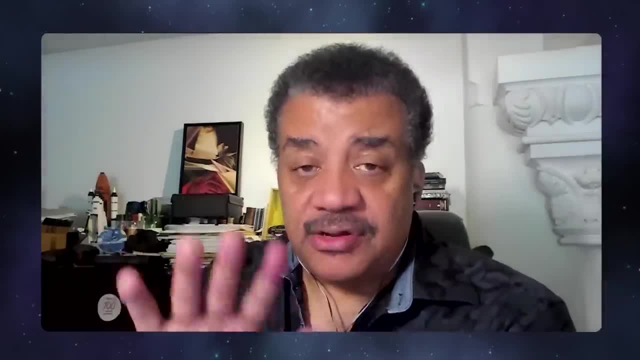 Right, Skin is very dark, It'll absorb most of them. That's because you know photons. they want to be a part of this baby. Let me get some. There it goes. Let me get some chocolate. Oh, I see where we're landing. 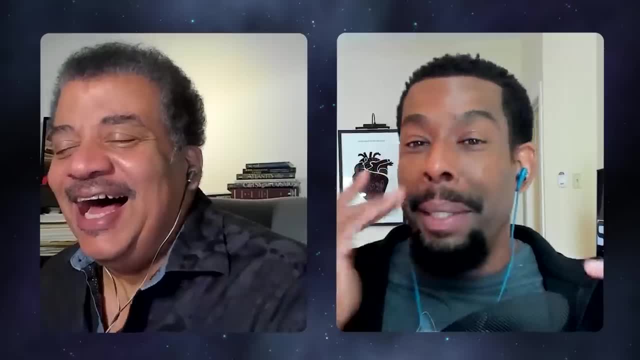 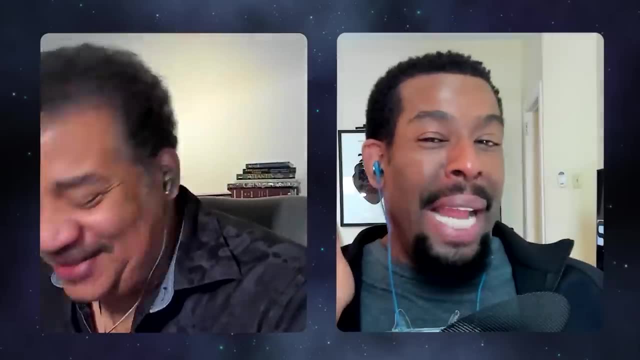 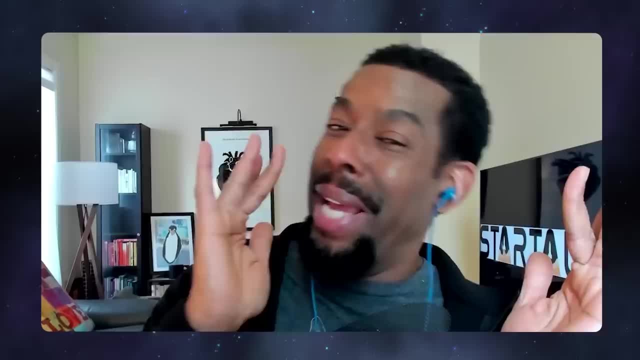 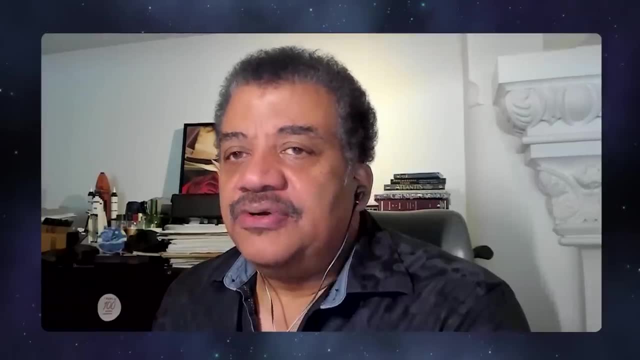 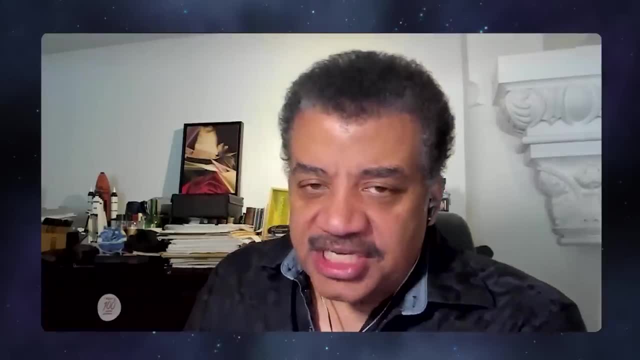 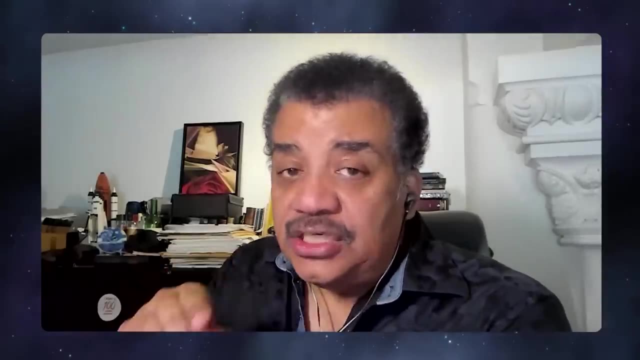 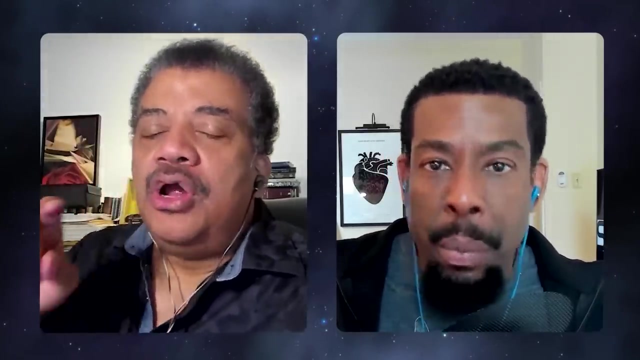 a microscopic particle. There's a particle size below which, when you open the curtains and shine light on you, that light will hit you and pop you into another location. So I'm smaller than the photon, Than what the Your Or what it. 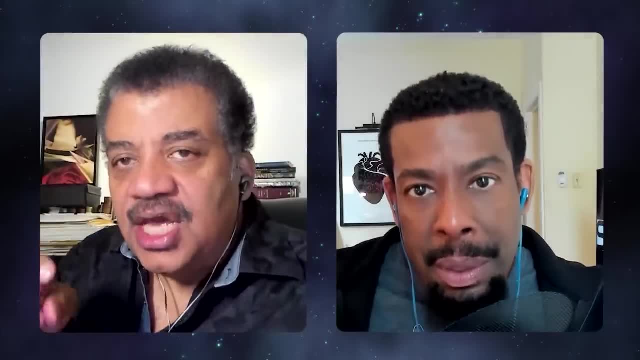 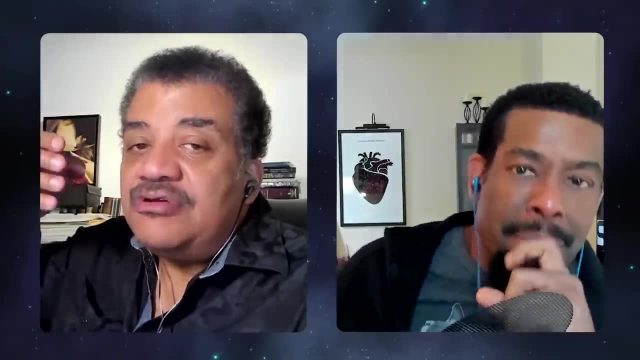 Your capacity to move to a different state of existence. That The energy that That is required. It's energy To make that happen. Correct, Got it. It's energy Is now the same as the energy of the light that's hitting you. 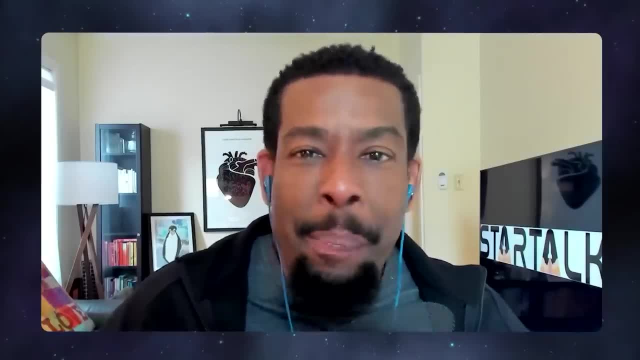 Gotcha. So you hit me with a ray beam In order to see, In order to see you, Right. And then you pop somewhere else And I say, where'd you go, Right? So What are you doing? 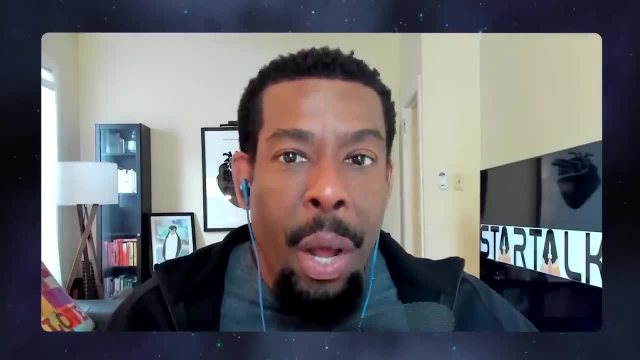 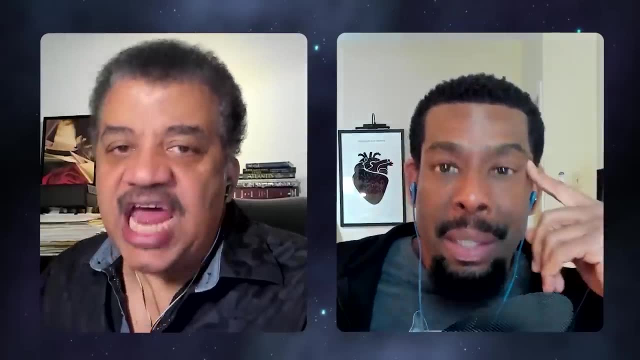 So am I there? Am I not there? Well, we'll never really know, because you're hitting me with something that makes me not there once you're exposing me to it. Correct, And since it happens on the moment you're exposed. 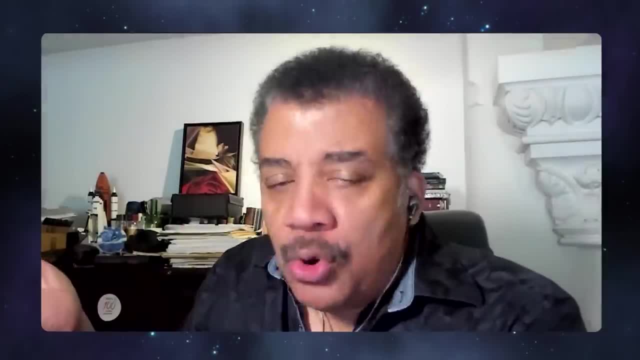 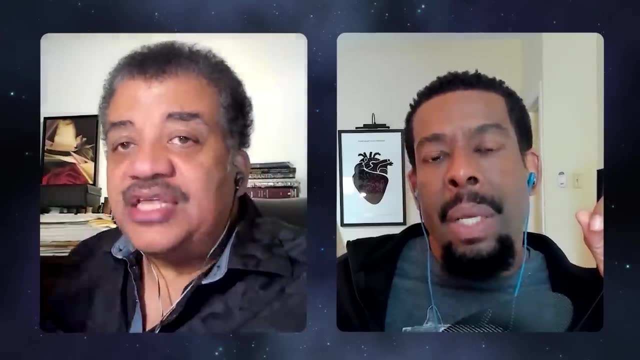 Right, Not the moment I see you, Right, I will never know what you were doing Exactly. Okay, If you're small enough for that light energy to affect you in that way. So that's why we don't think about this in everyday life. 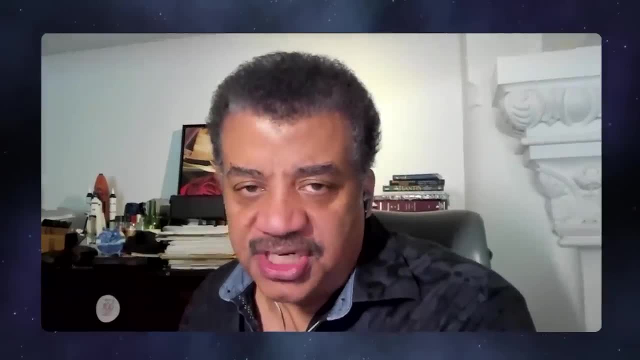 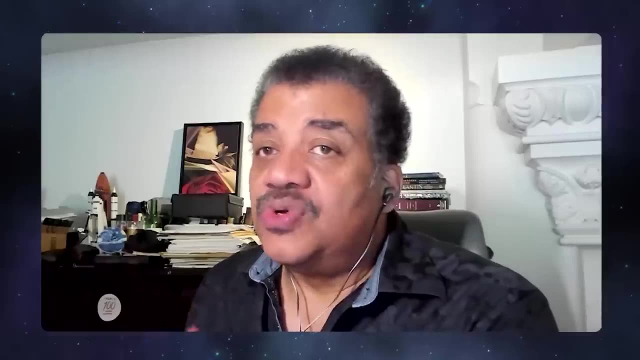 Because we're too big for light to pop us into other states of existence. Exactly, But particles, electrons, atoms, nuke, all of this it happens all the time, And this was a very disturbing discovery in the 1920s. 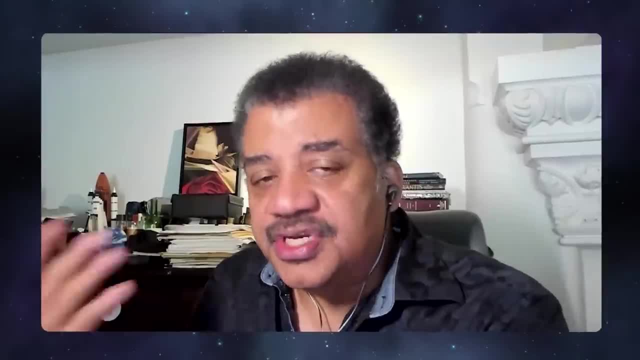 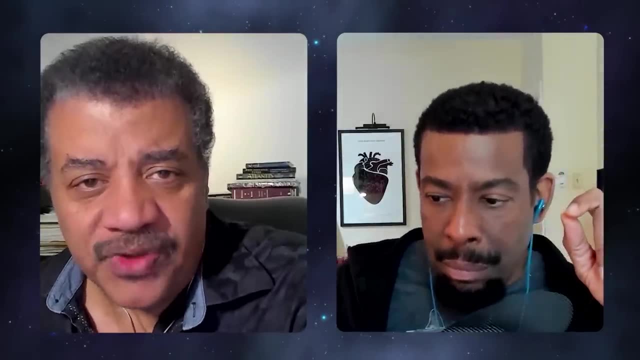 We're in the centennial decade of the discovery of quantum physics, in the 1920s, Because you discover: I wanna see what you're doing. Oh, my gosh, you're not gonna let me see what you're doing, Because the light I shine on you in order to see it is. 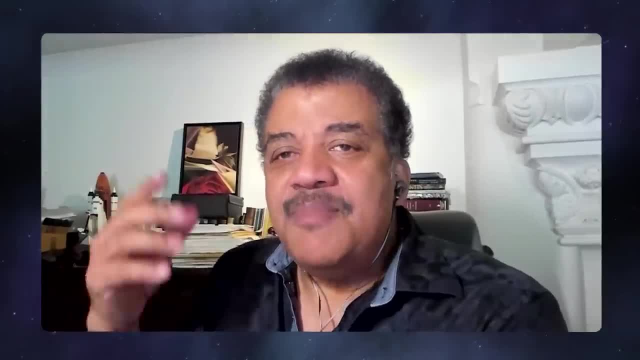 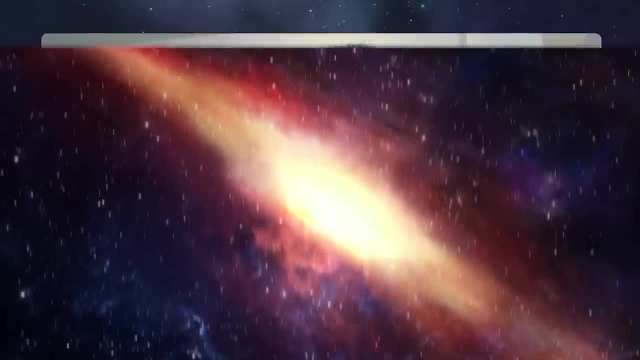 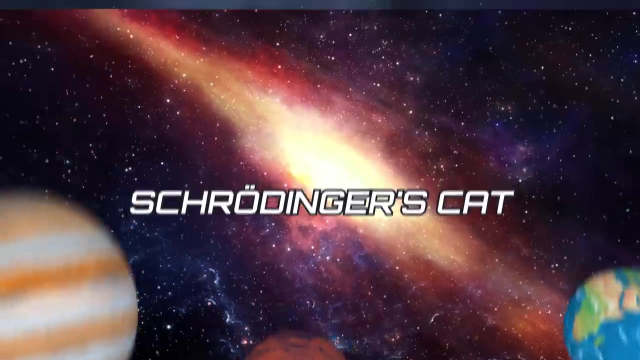 So it's really. It's not so much an observer effect, it's a measurement effect, Exactly Okay, Get the human brain out. It's just a device to measure you. You can't know it, Okay, Right. So here's what happens. 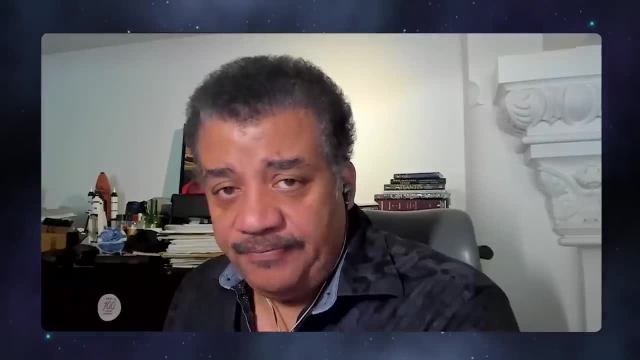 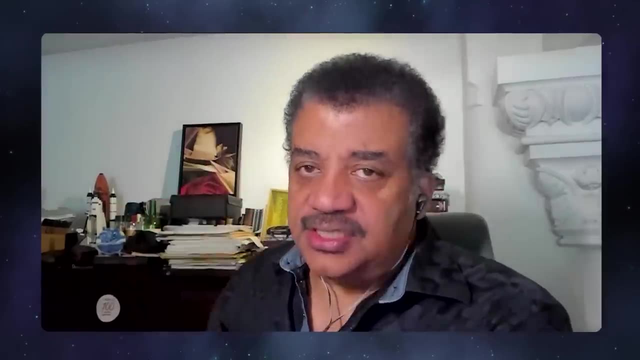 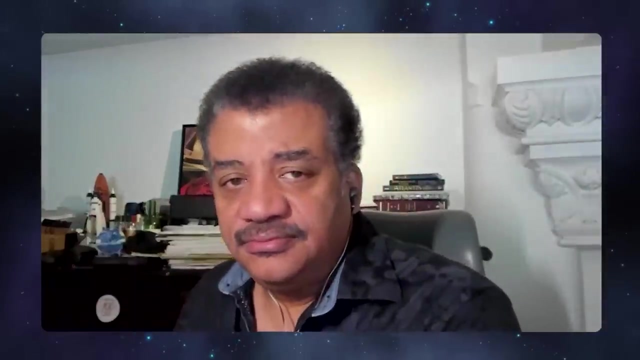 You say to yourself: you put a cat in a box, And if the cat is a quantum cat with two states, states of existence, it's either dead or alive. while it's in the box, you have no idea which it is. 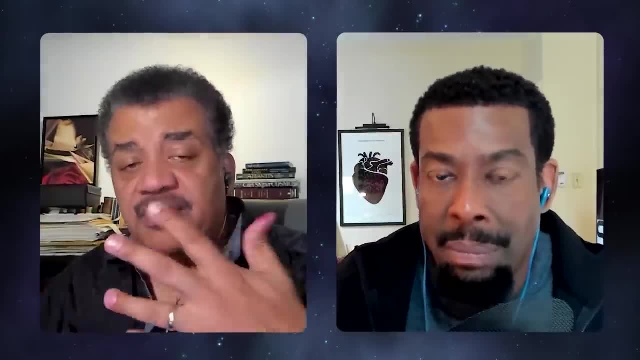 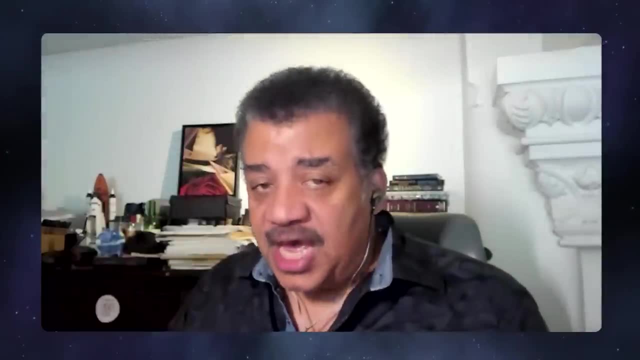 And so the way we describe this in quantum physics: if you do the experiments, okay, so some percentage of the time, Okay, You open the box, the cat will be alive, others the cat will be dead, And so you. 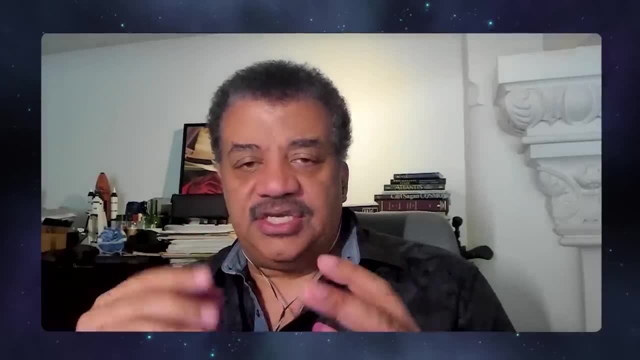 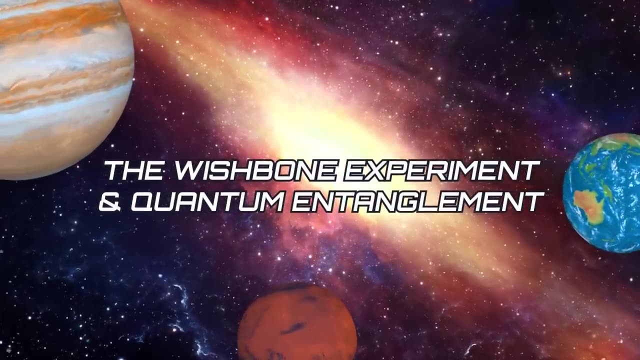 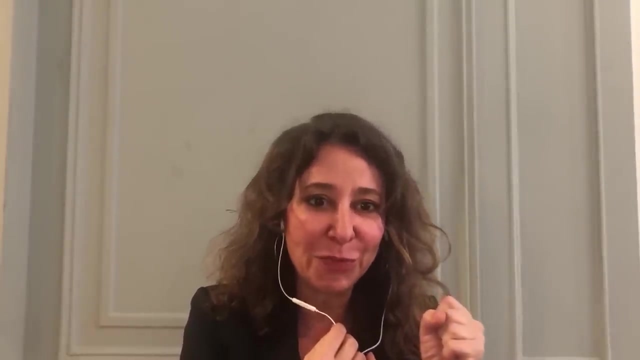 What we say is that the cat's existence is a superposition of being dead and being alive. So the wishing bone experiment, It's the wishing bone experiment. Okay, So we break the wishbone in half. We don't look at our pieces. 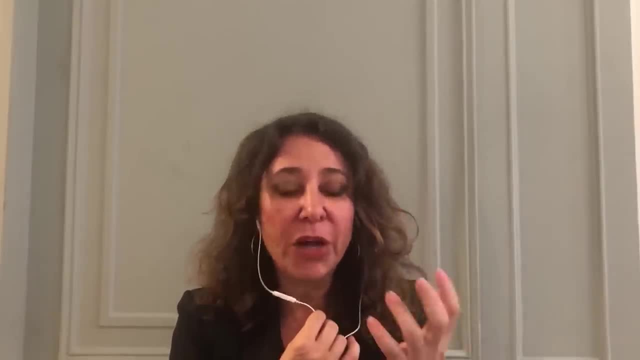 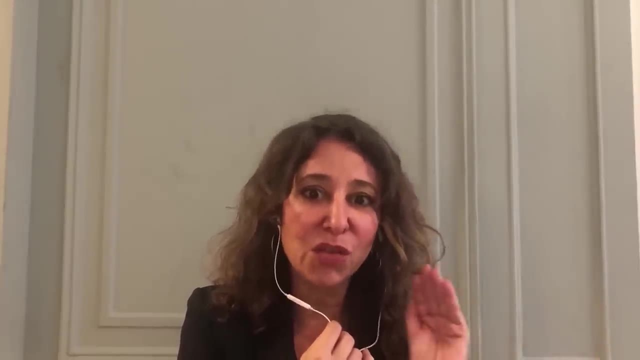 One has a big piece, one has a small piece. I go to Andromeda, I look at mine And I find out I have the big piece. I instantly know: you have the small piece. Now, there's nothing surprising about that, because it was established at the table which. 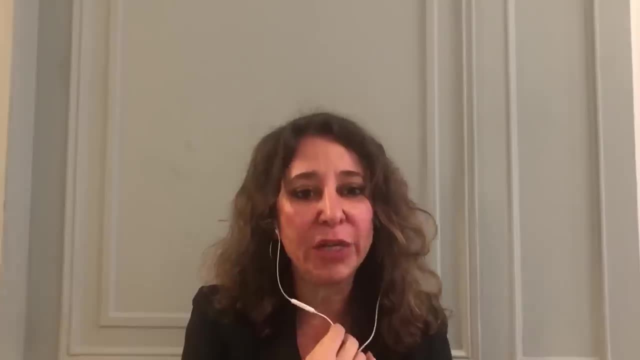 one had the big piece and which one had the small piece. Right right Now, quantum entanglement is much weirder. It says we break the wishing bone and it's simultaneously in a state where I have the small piece, you have the big piece, and I have the big piece, you have the small piece. 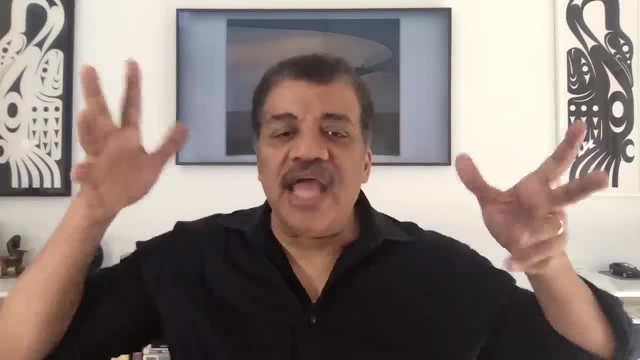 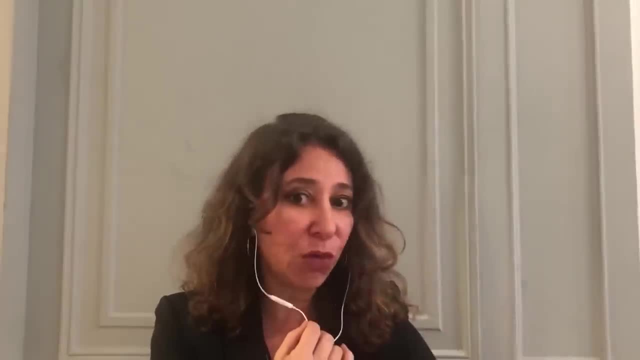 Right, It's indetermined By any entity. No, It is completely in what we call a superposition. But it has to match. We can't both have the small piece and we can't both have the big piece, Right? That's why the two states are not. we both have the big piece. 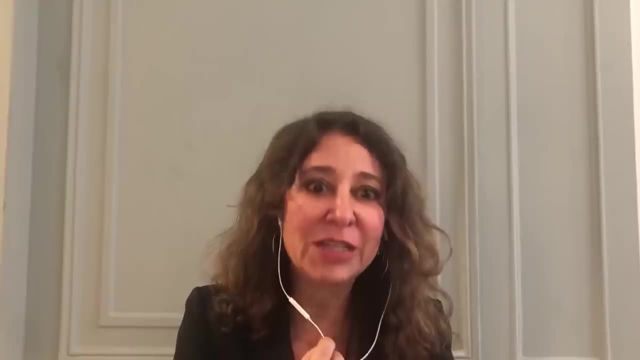 It's I big, you little, You big, I'm little. Right, It's the two states Exactly. But they have to match because they have to fit together to make the original wishing bone Right. But it's not actually determined who has the big piece yet. 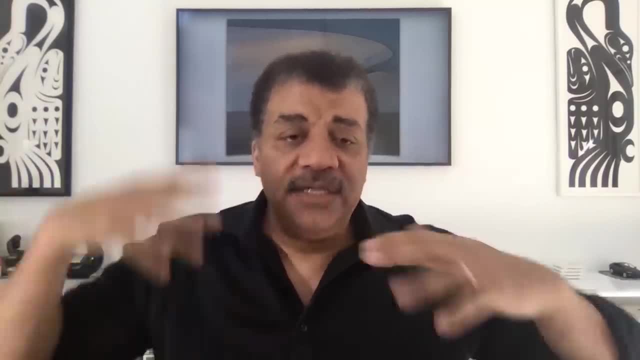 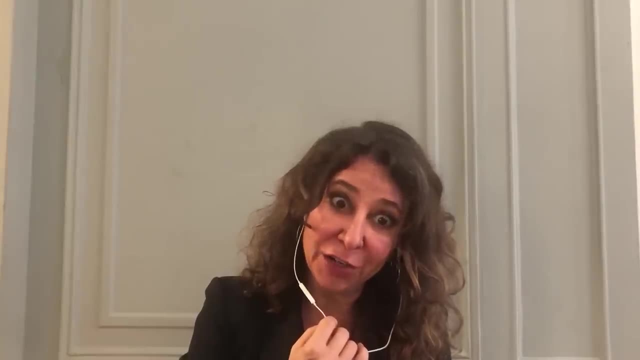 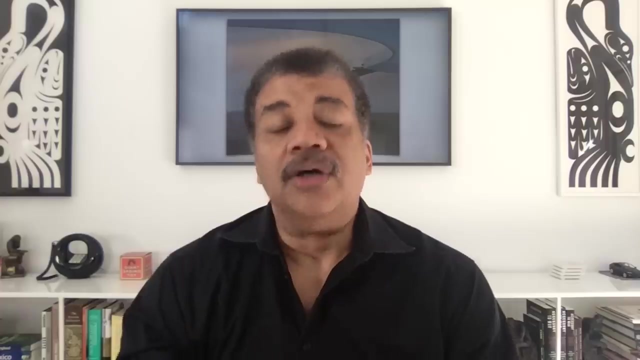 Right, And quantum mechanics allows for this. We can't know. Is there some higher dimension? Is there God, who would know? Well, if you're real adherent to quantum mechanics, you would say that you've disproven the possibility of omniscience being. 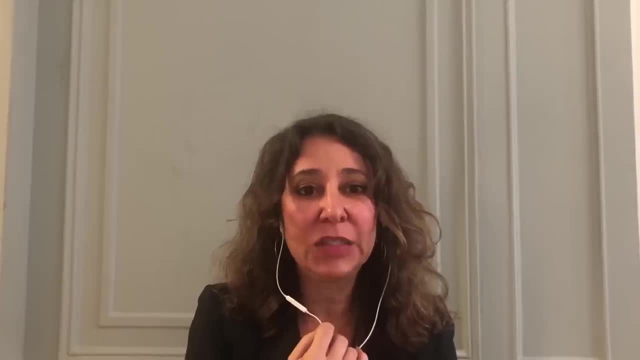 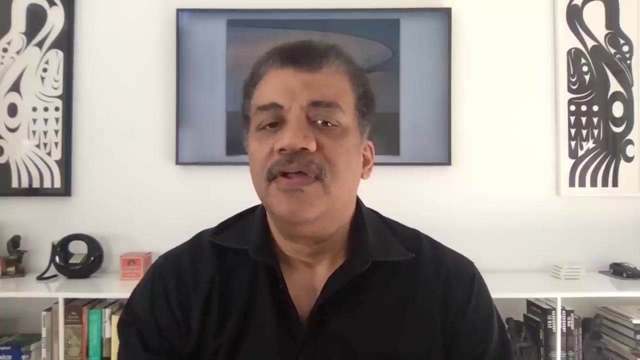 Because, no, it is not established In some sense, when we, in our conventional thinking, are accustomed to thinking certain things are real. What's real is: the piece of the chicken bone is real, We're sure of it, But it's not in some sense real. 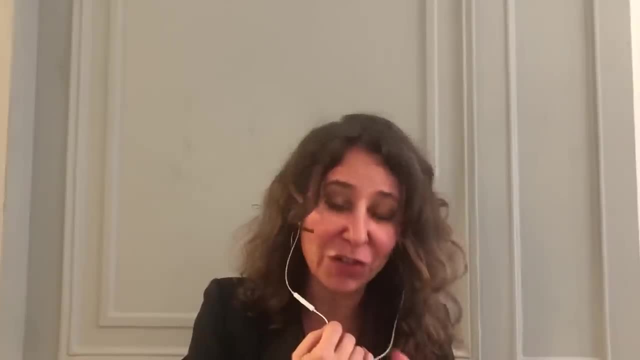 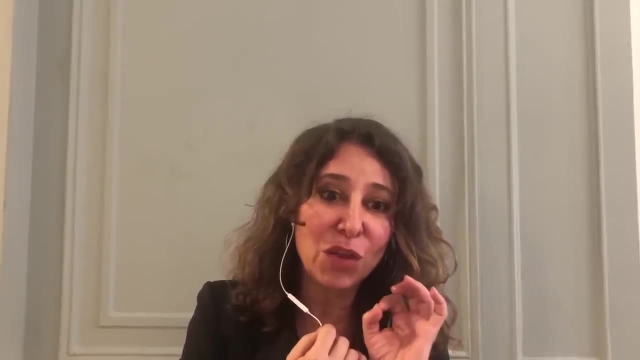 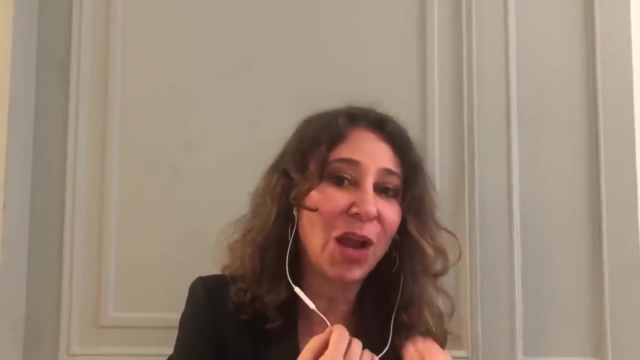 What's real is the probability. that's real and that's determined, and that is absolutely deterministic and can be predicted. the probability But the existence of the pieces of bone themselves are not yet actualized. They don't actually have a concrete existence. Right, 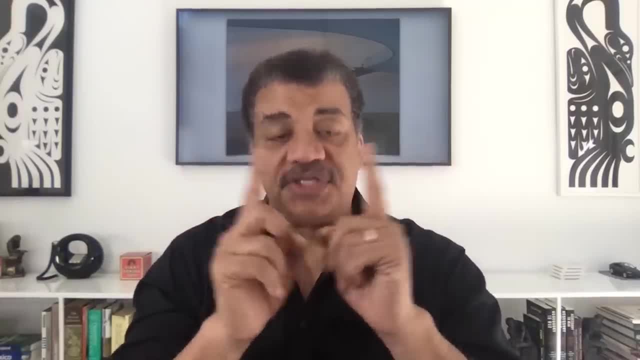 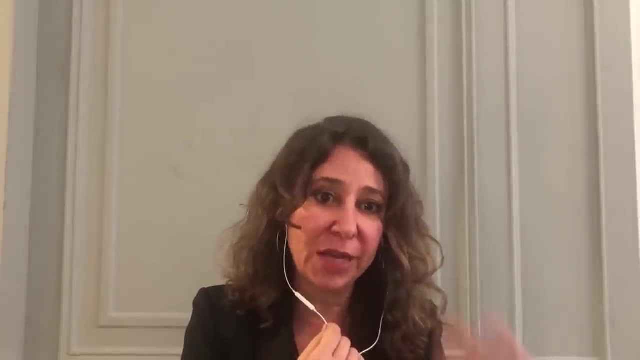 Right, You and I are entangled with each other, Right, And we have to be entangled because we can't both have the small piece, because that's not cool. So we have to be entangled in such a way that we fit together correctly to make the original. 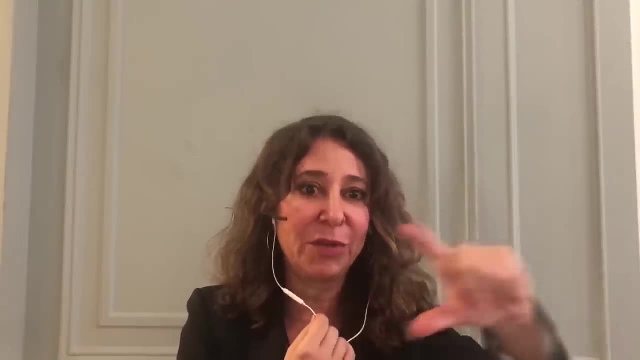 wishing bone. So I can have the small piece, You could have the big piece. I could have the big piece, You could have the small piece, But we don't know which one it is yet. It's not just that we don't know. 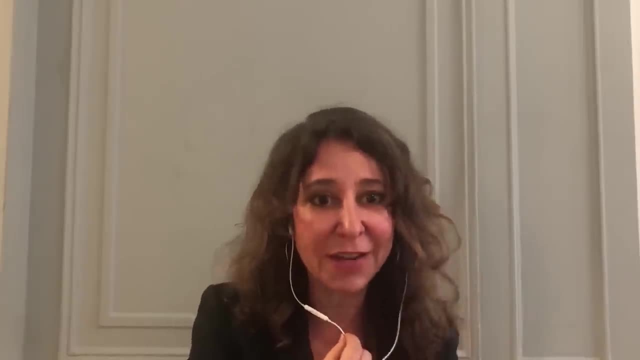 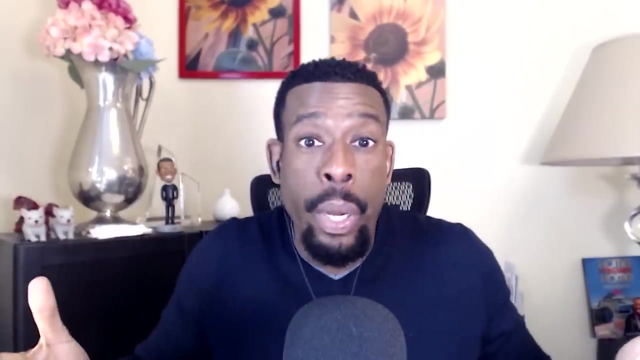 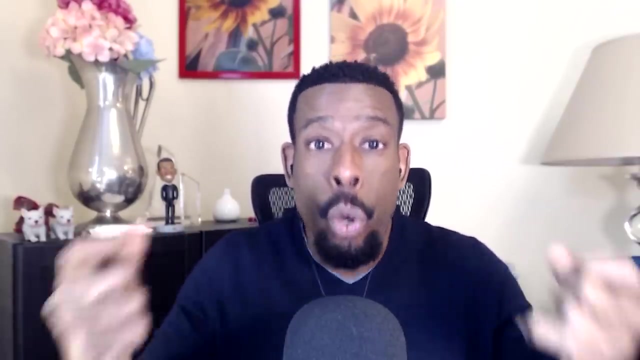 It's that it doesn't actually assume a precise sequence. It doesn't assume a precise state yet. Okay, So when does it assume that precise state? Because at some point this can't just be potential. At some point there has to be a realization of who has what piece. 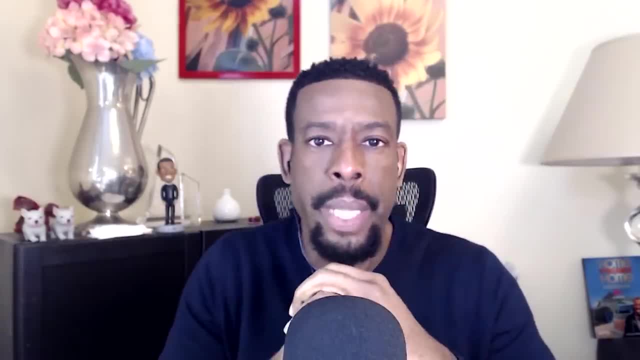 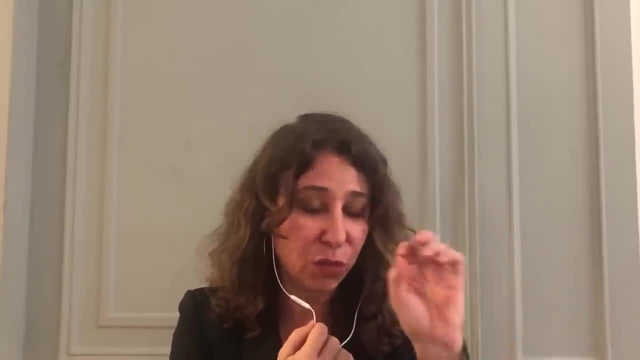 So when does that happen and how do we determine that and how do we observe that? So superpositions are very delicate. So when they do it, as you were saying, Neal, like in the laboratory, everyone's trying to do this in the lab. 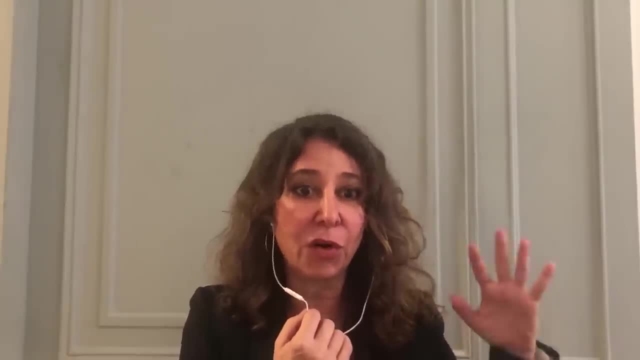 It's very, very, very delicate. You have to have systems that are not disrupted or disturbed in any way. So there was this sort of mystique that once I went to Andromeda and I looked at it, that the act of my conscious looking forced it to assume a certain state. 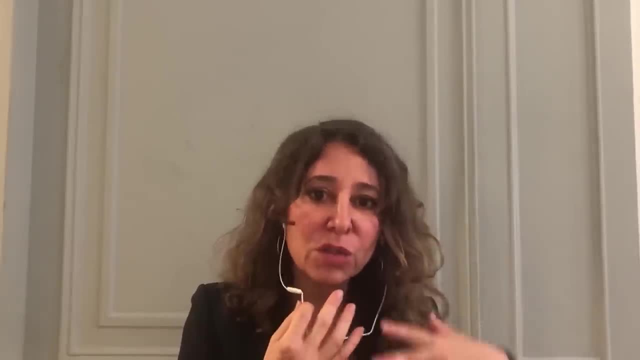 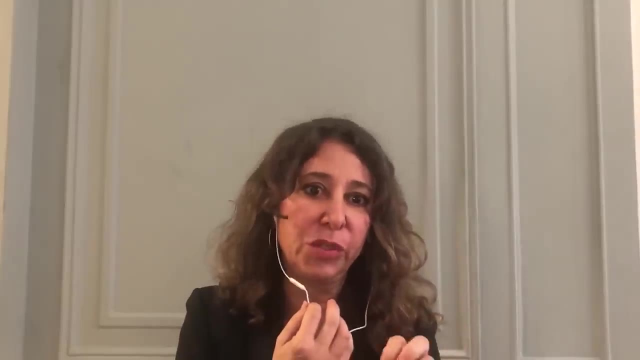 And that's not really quite right. What happened was just all the molecules in my body and the air that I'm breathing and the room. all of these things destroy the delicate superposition. They knock it about. Imagine, you know, a pencil standing on its end. 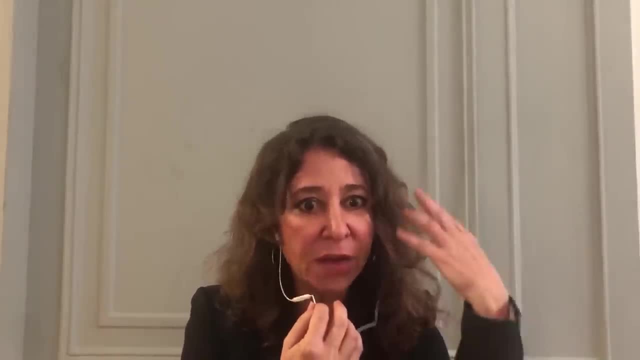 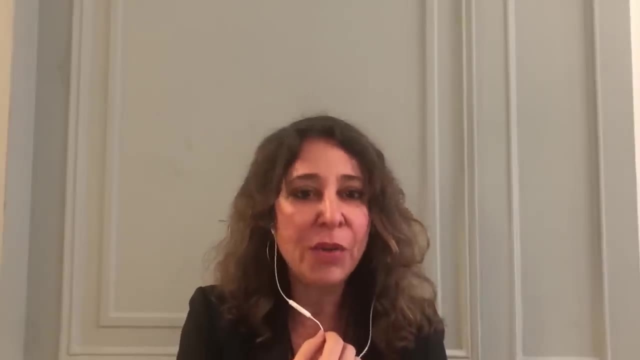 So yeah, if you go and clumsily look at it, you knock it over. But it doesn't have to do with your consciousness, It's just the interaction of all the particles and all the molecules and all those things that make it impossible for it to maintain this delicate state of standing on its point. 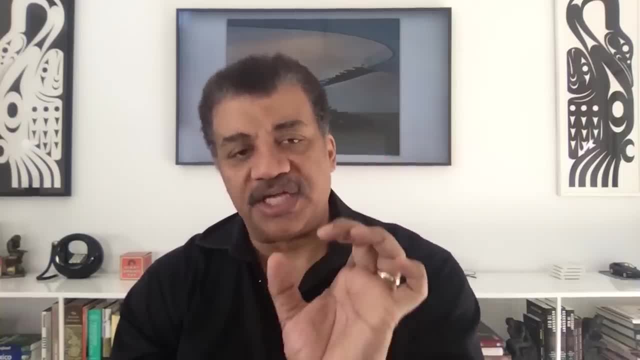 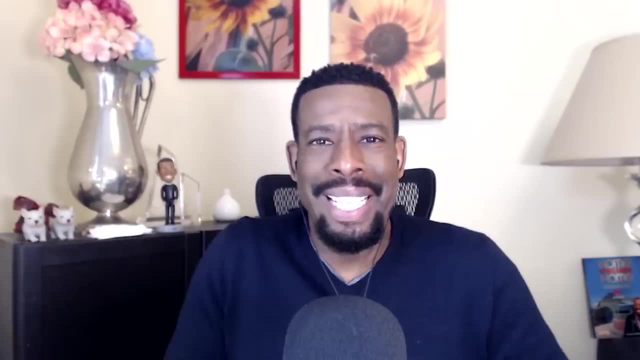 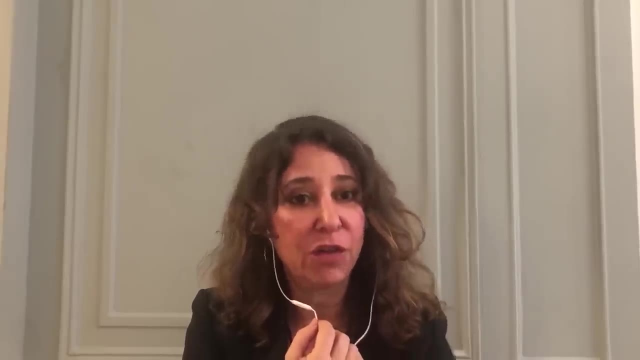 Okay, So now the state becomes actualized in front of you. Yeah, So now I look and I know for sure I've got the big piece I won. But what happened? is I somehow seemingly forced faster than the speed of light from Andromeda? 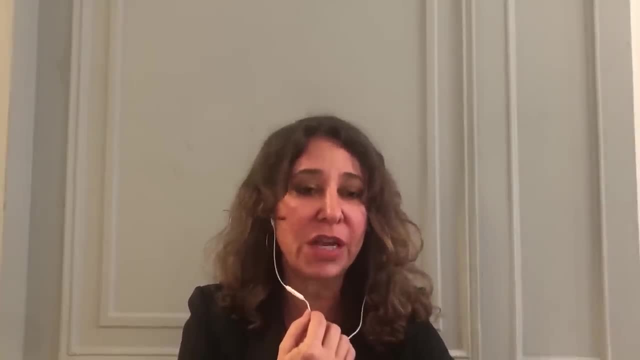 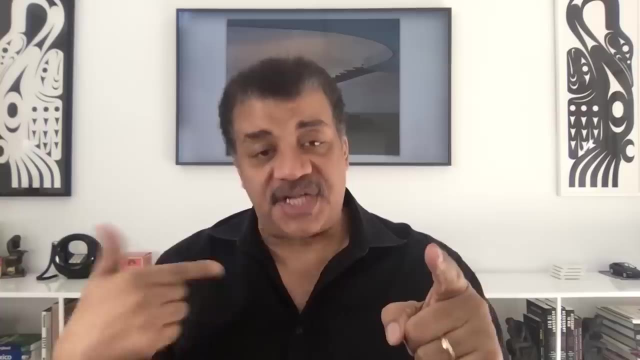 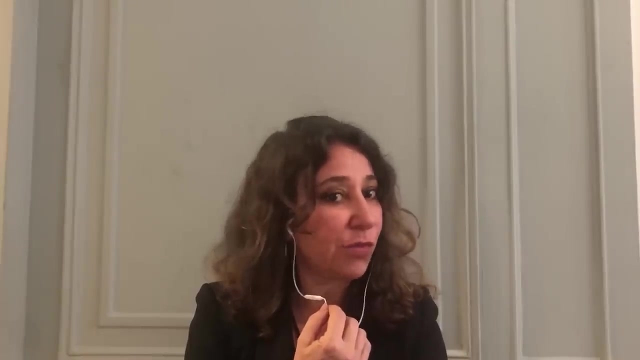 to the earth instantaneously forced your state to also assume a precise state, Because you can't know that without me also knowing my state Right. Well, I can look at it and know it and I instantaneously know you have the small or 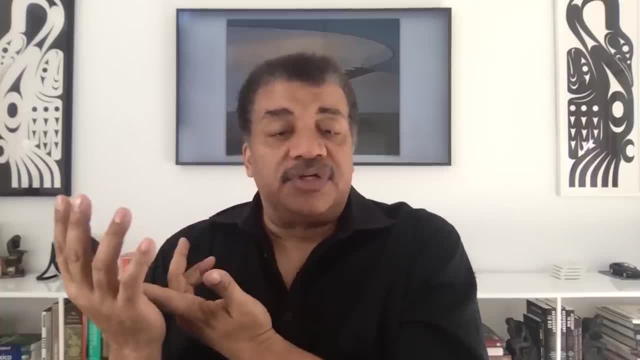 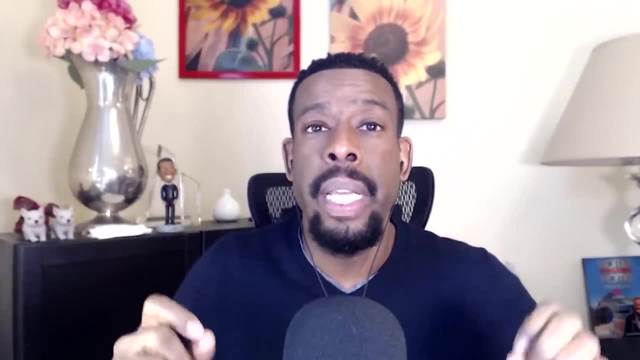 the big piece of bone, and that's that. But you don't necessarily Whether I've looked at it yet or not. That's right. But that's only because there has to be that balance of big and small. That's right. 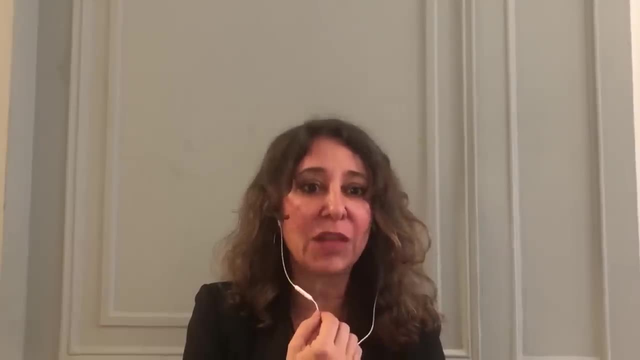 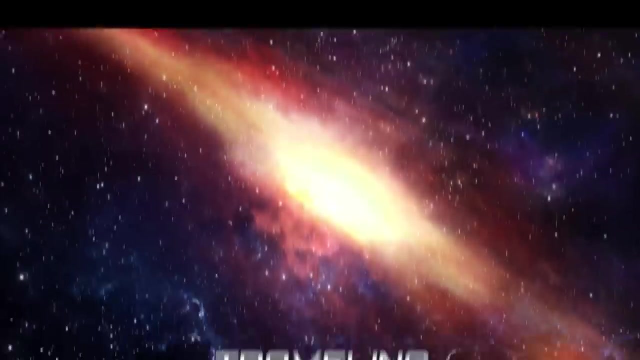 Exactly. That's the only reason, Right, They have to fit together to make the original wishing bone Exactly. It can't be that I look at mine and then you also look at yours and we both have a big piece of wishing bone. Theoretically, Dr Tyson, do you think a superhero with the power of inter-universal travel could ever be truly possible, Or would the probability of the laws of physics in other universes being different from ours prevent that from ever happening? Could somebody do it? 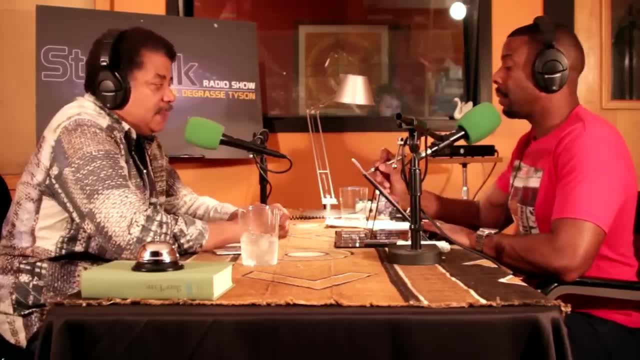 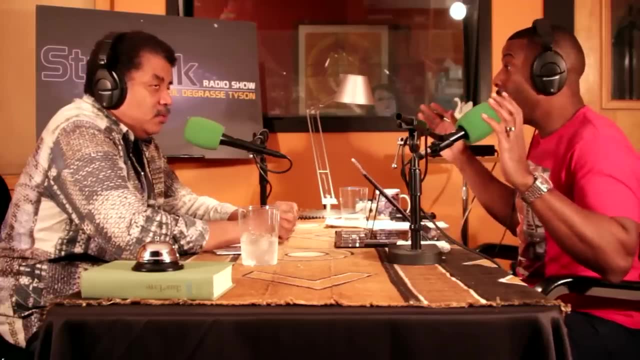 Awesome question. So in the multiverse concept, Yes, Which, by the way, in Thor, that is what happens. It is the inter-universal, Inter-universal travel, Because Thor opens No way From his world, opens up a portal. 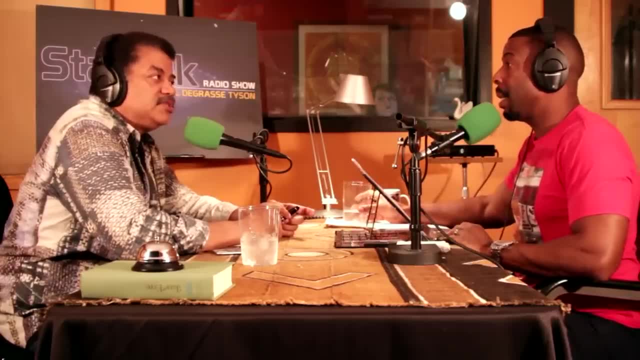 No, no, no. His world. I think his world is in our universe. He just The portal gets you from his world to our part of the world. Oh, okay, All right. So there you go. Isn't that world sectors? 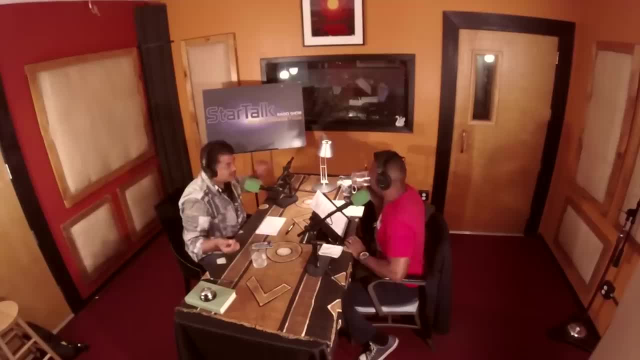 And we're one of those sectors. I think it is. I think you're right, You're right. There are six sectors, Right, Exactly, And we're one of them. We're one of them, And so this is easy access from one sector to another. 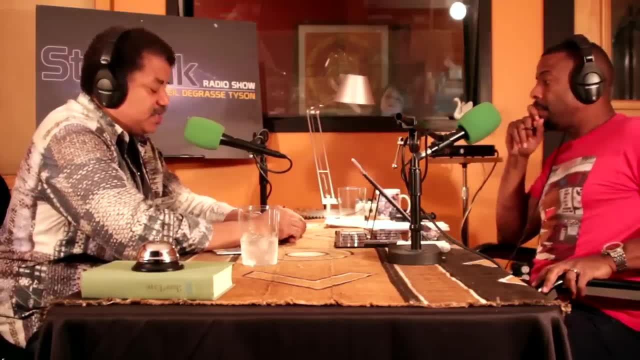 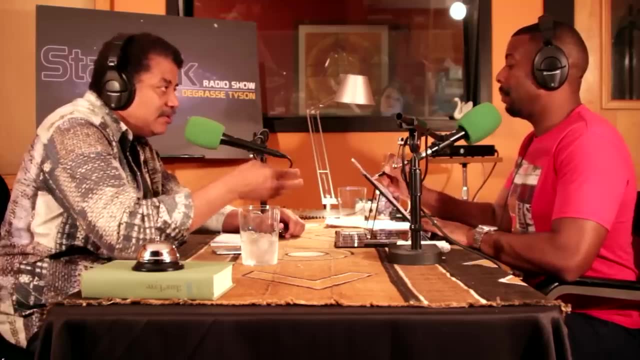 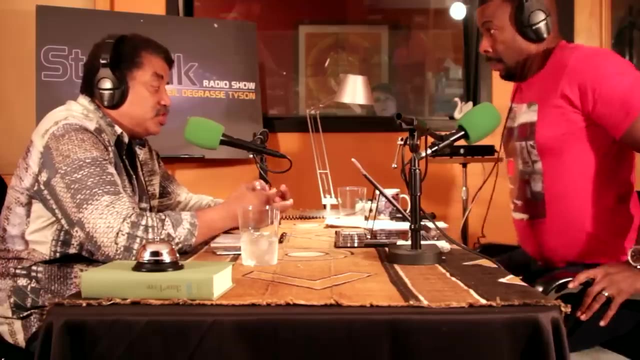 So that's a wormhole, That's a wormhole, It's essentially a wormhole, But this would be an inter-universal portal from the multiverse. It's prescribed by the fact that these are fluctuations in the early quantum universe, And quantum physics is a fascinating understanding of the structure of matter on the smallest. 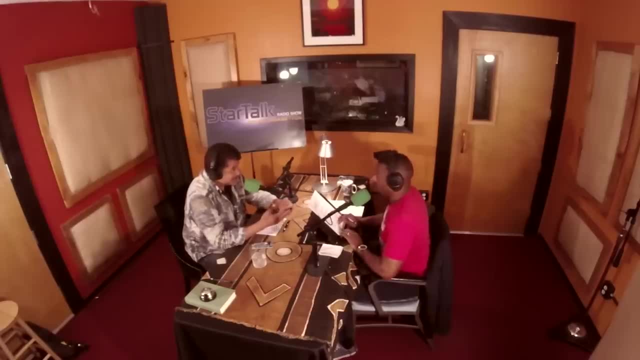 scales Right, There's particles that pop in and out of existence. I mean, it's a stunning reality that exists at those scales Now the whole universe doesn't do that, unless the entire universe were the size of an atom. Then when you pop particles in and out of it, 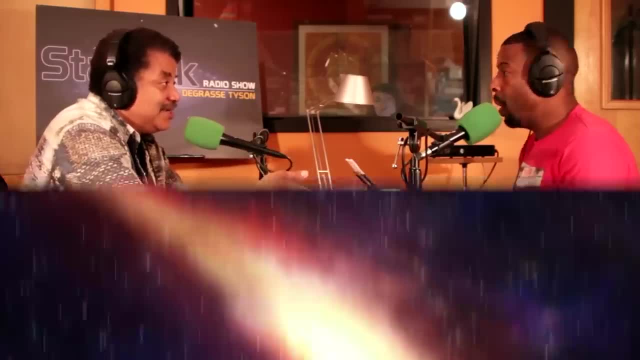 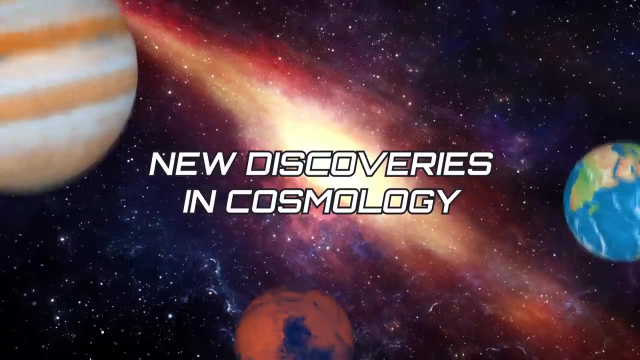 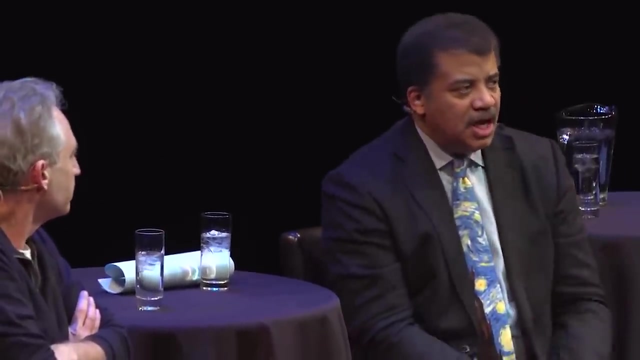 When you pop particles in and out of existence, you're actually popping universes in and out of existence. Whoa, Whoa. What I'm asking you as a theoretical physicist, leading theoretical physicist: we have an observation, an astronomical observation, and it forces you to go back and re-tweak. 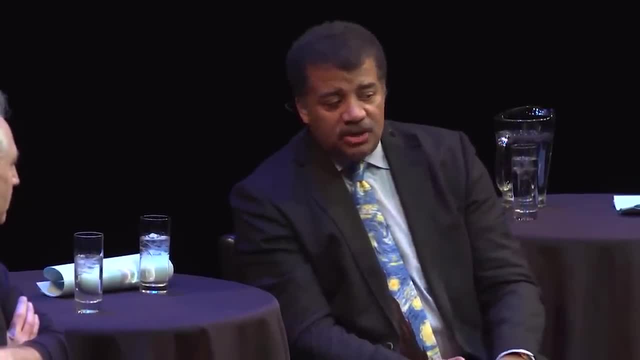 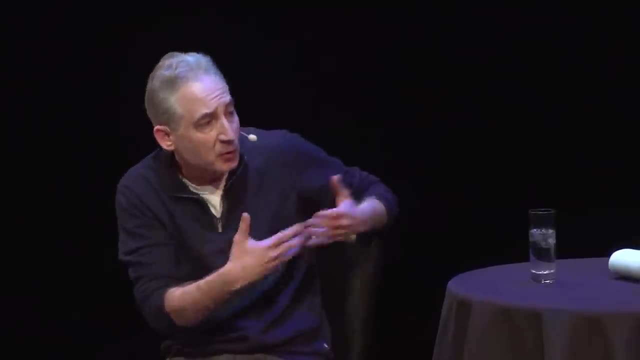 You're tweaking Big Bang. You're tweaking quantum physics. You're tweaking What are you tweaking? Well, in this particular case, you really are tweaking What? Something that we yet don't understand fully, which is dark matter. So that's right for being tweaked. 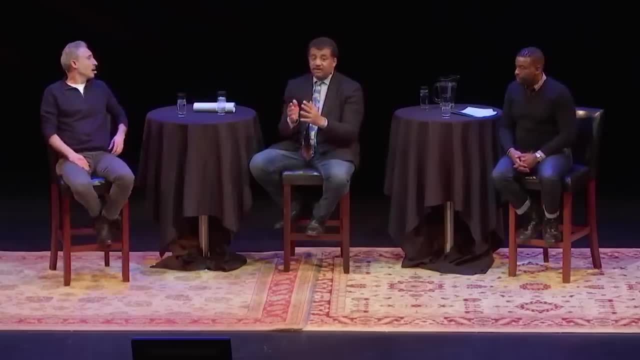 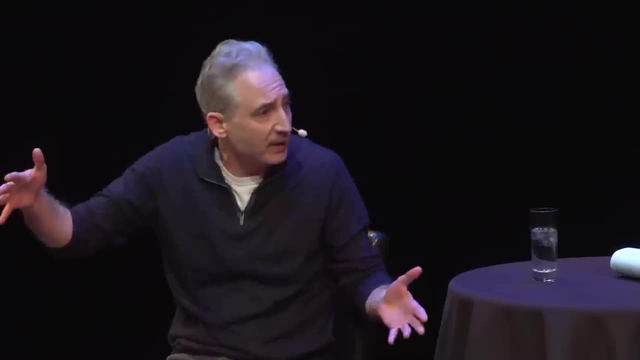 But look, there are other things. So dark matter is like mysterious gravity of the universe and we have no idea what's causing it. But I'll give you another example which has happened recently. right, There have been measurements of the rate of the expansion of space. 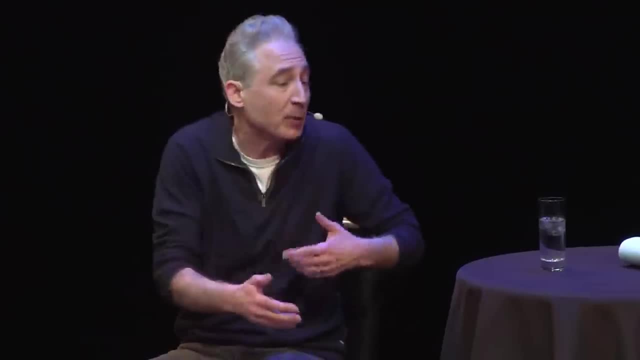 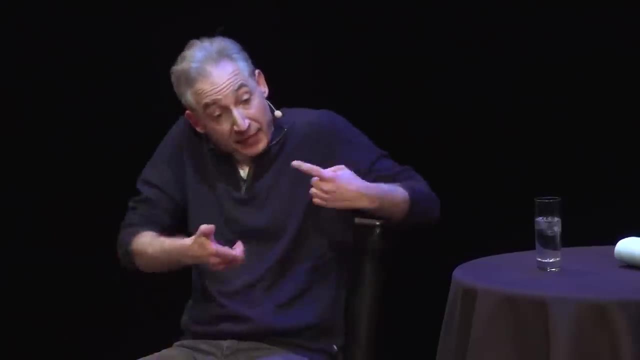 And those measurements, very recently, are seeming to be incompatible with earlier measurements done in a different way. This is yet a whole other recent result, A whole other recent result, Exactly, And this one, if it's correct, this is one that could really change our understanding. 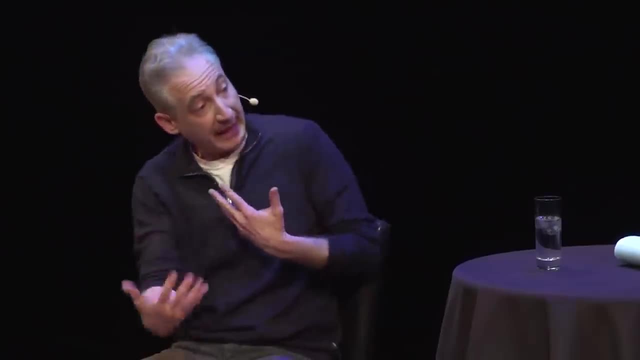 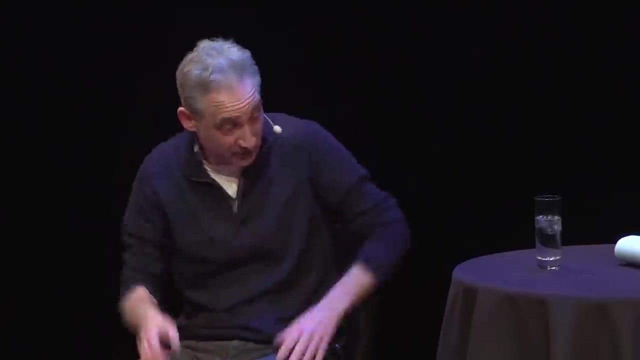 of the early universe dramatically right In order to get the measurements that are done on the expansion of space, looking at the microwave background radiation- and those that are coming from looking at supernova explosions. to get those compatible right now is going to require perhaps tweaking the 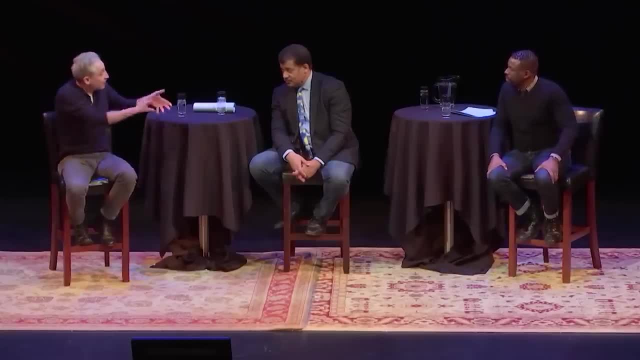 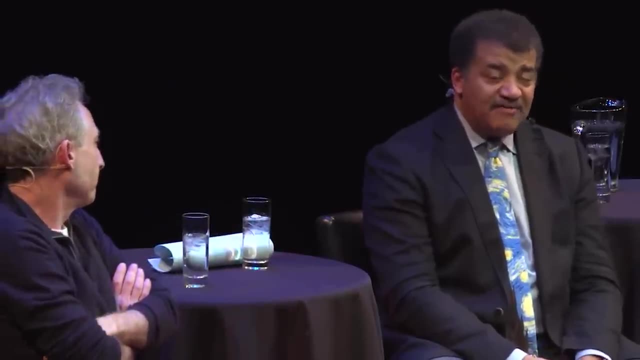 dark energy. It may require tweaking our understanding of the gravitational force. I mean, there are many things that may come into that particular Tweak our understanding of the gravitational force itself. Yeah, I mean whenever you talk about dark energy, right? 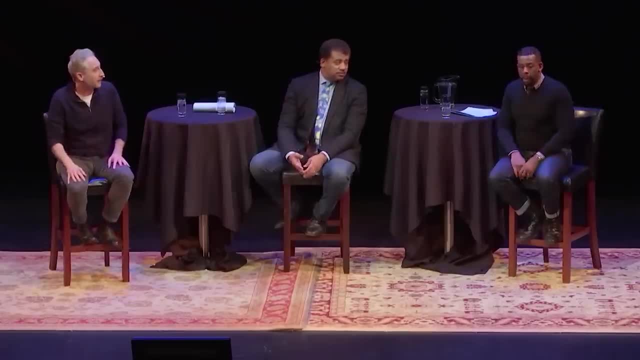 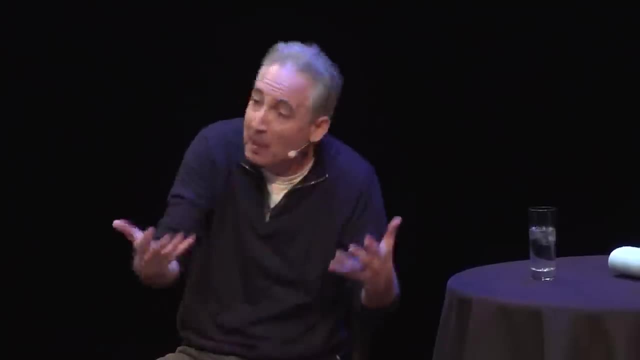 Everyone knows what dark energy is. Yeah Well, I'm just saying, some people at home may not, Right? So this energy-filling space that we believe yields a repulsive gravity that's causing the universe to speed up in its acceleration, and 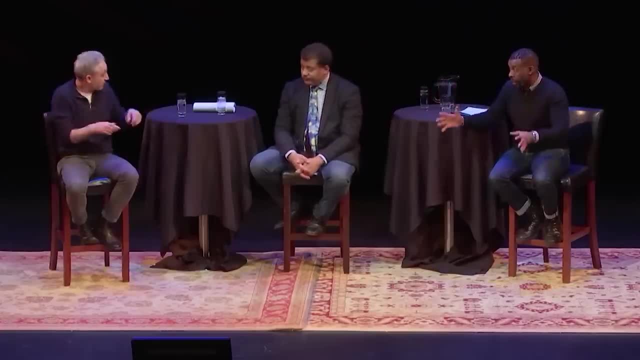 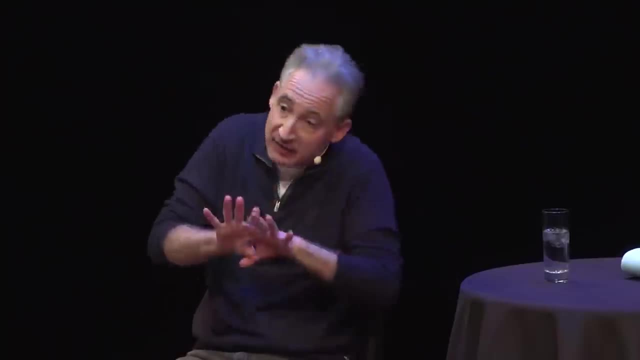 When it theoretically should be slowing down. That's right. Ordinary gravity pulls things together. Right, It should be slowing down. Okay, The shock that we got in 1998 is that it's not slowing down in the rate of expansion, It's speeding up.